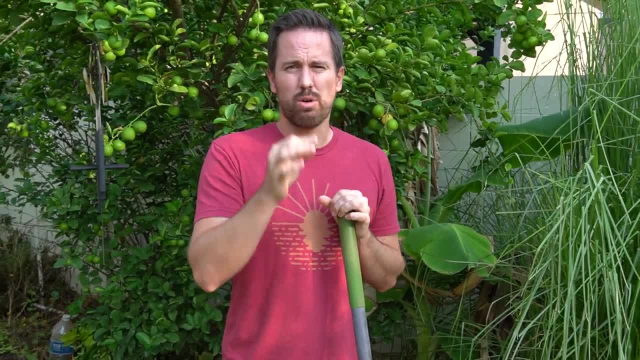 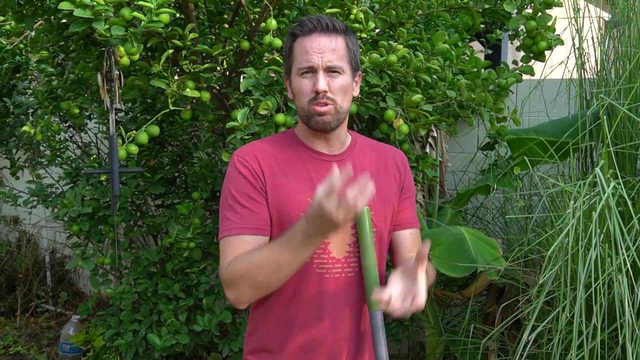 at least the way I like to do. I never like there to be more than three or four pups or stalks growing at the same time. The reason for that is because if you have too many more than three or four pups growing, the corm or that underground system is not going to be able. 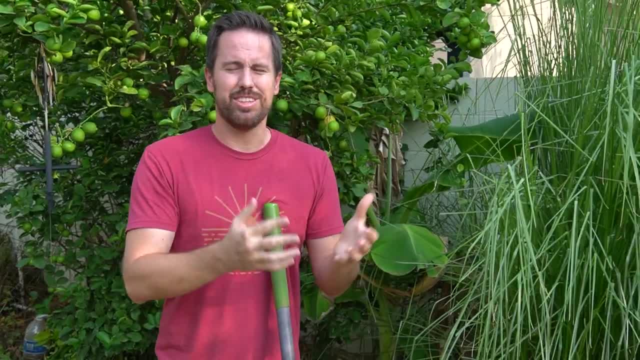 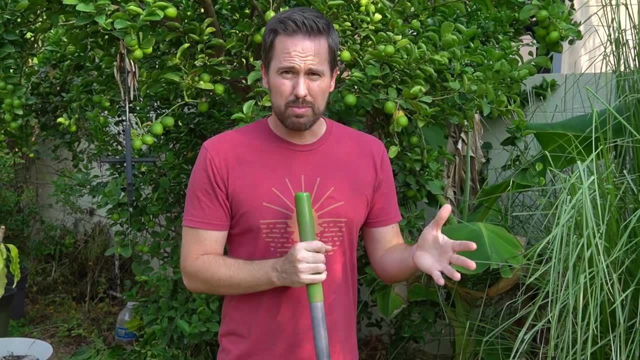 to supply enough nutrients to grow big, awesome, nutritious, healthy bananas. So never allow more than, like I said, three or four pups to be growing. One cool thing about this is, once you have one banana plant, it's going to produce enough pups to where you can cut them out. 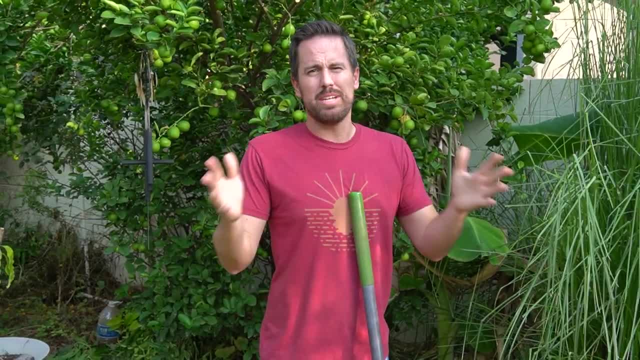 propagate them, plant them over there. plant them over there. plant them over there. After a few years, you have more banana stalks, more banana trees, and you know what to do with it. Okay, so now let's get in here. 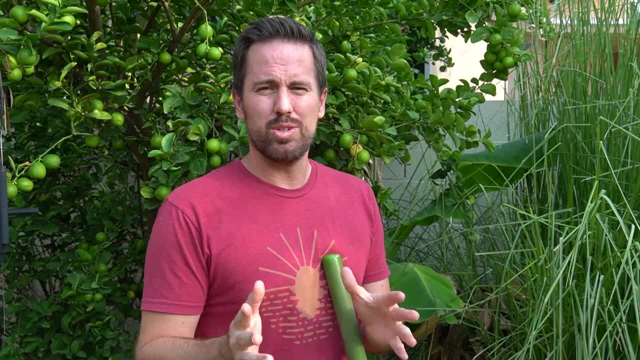 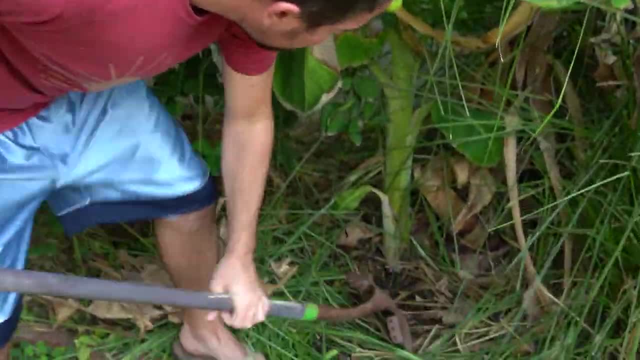 I'm going to show you how I cut it out. It's actually very simple, but I want to give you the visual so you see it, so you can go and do it on your own. So if I get in here, the mother plant is actually you can see the old stalk that has since died, but it's right. 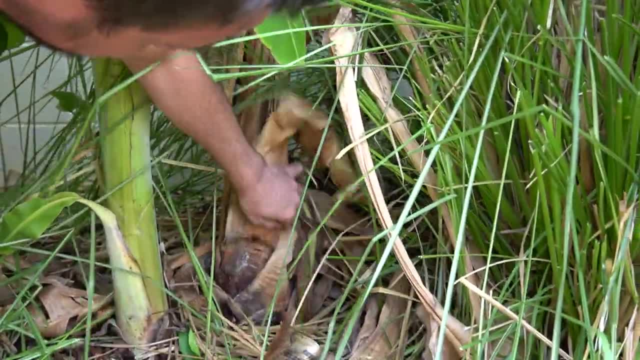 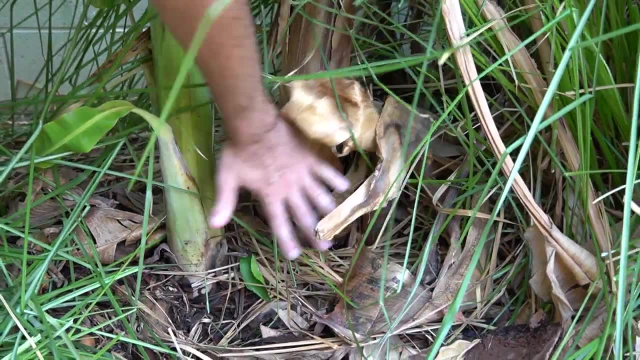 here And there's actually you can see there's another pup coming up right here. It's very small. It looks a little rotted because we've gotten lots of rain lately, but it's right here. So I know that the corm is over in this direction. So what we want to do with this pup right here? 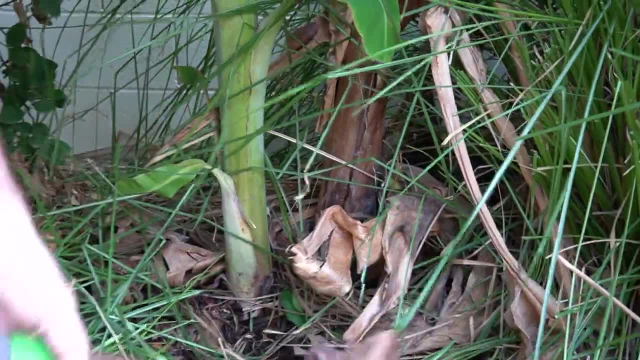 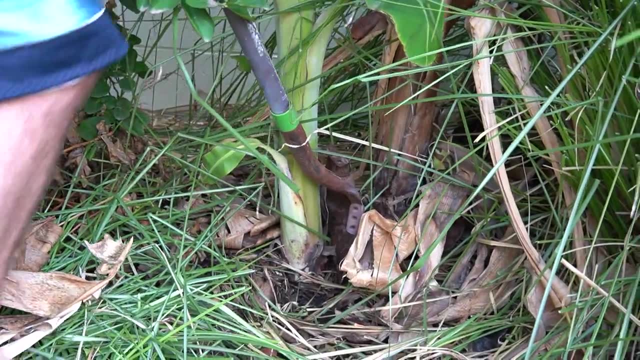 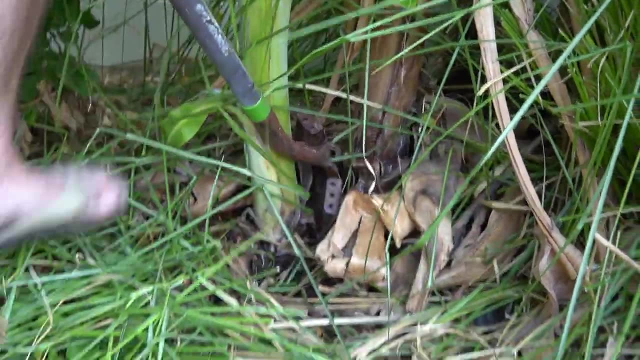 is, we want to separate it from the corn And we do that by simply cutting it out with the shovel. So it's a little hard back here because there's not a lot of space, but I'm just going to put my shovel right in between And without hitting, not too worried about the old banana stalk, because 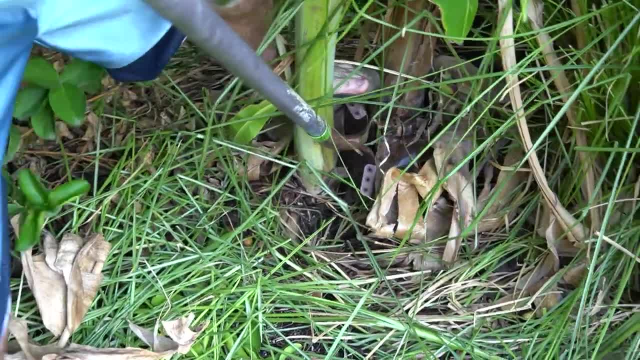 it's gone and dead, but I'm just going to cut down in here until I get through and slice that corm out. So that's what I'm going to do. So I'm just going to cut down in here until I get through and slice that corm out. 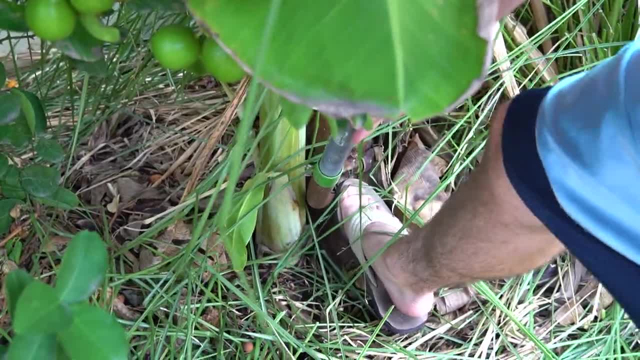 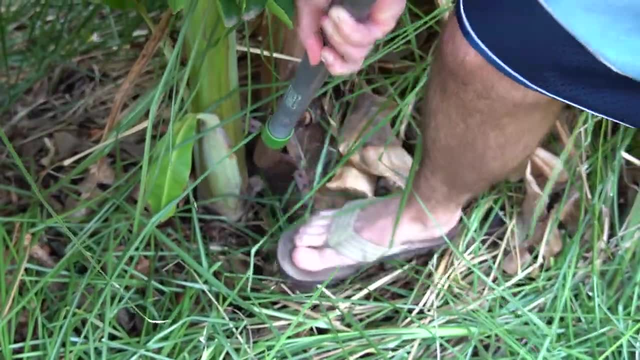 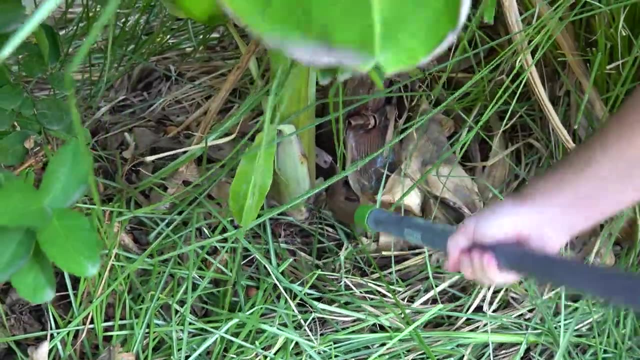 You can hear that once I got through the corm you could actually hear it snap. This is a better angle for me to get down in there. Once you separate that corm it's actually pretty easy. You can see there it's already moving. 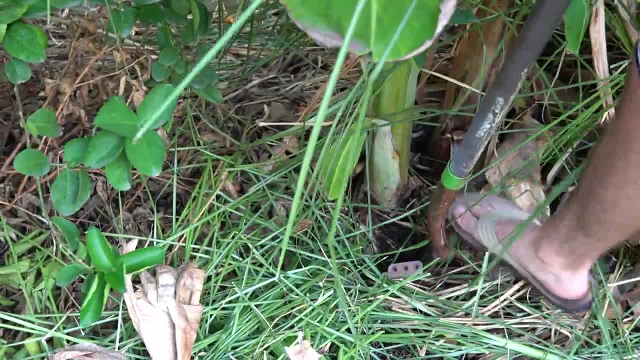 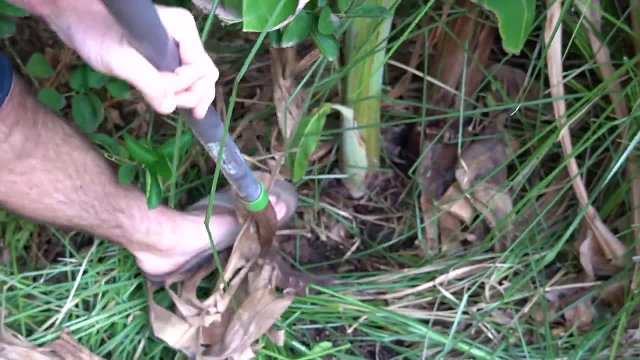 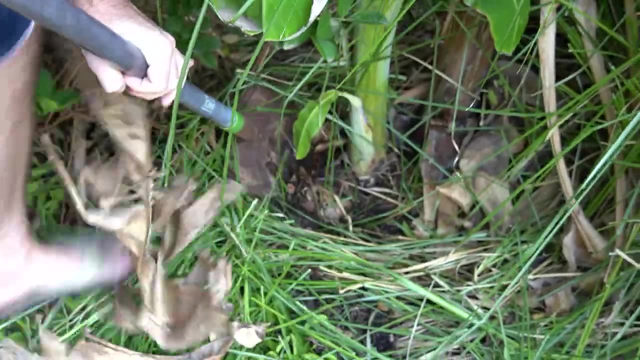 So then from there you just slowly go around and underneath the whole thing So you can see there it's already moving. So then from there you just slowly go around and underneath the whole thing thing and we're just slowly digging it out there's. it's connected to the corn. 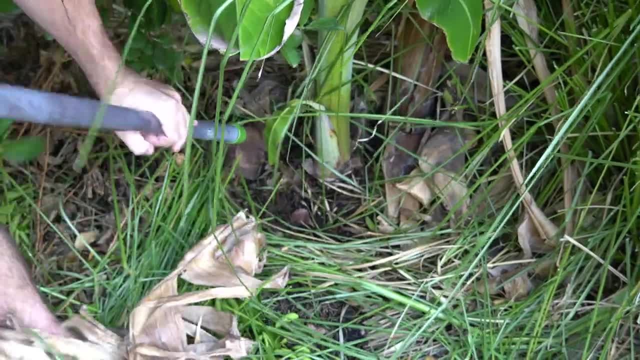 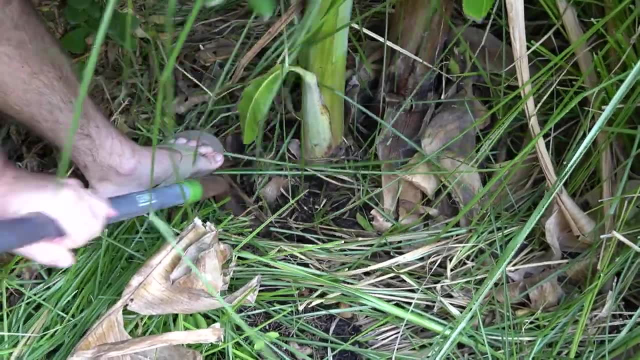 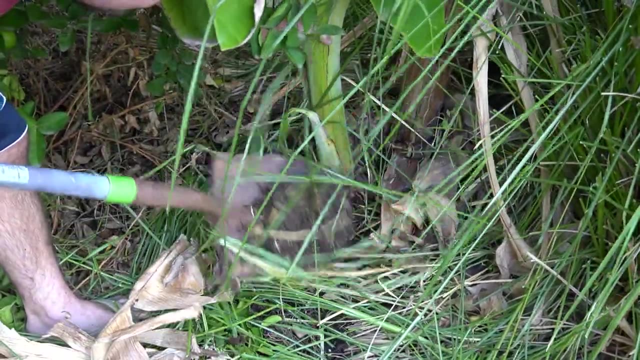 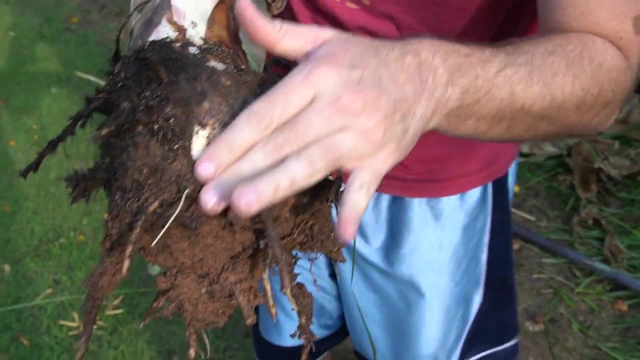 but it also has roots that it's spreading out as well, and if it wasn't back here in such a tight space, it would already be out. boom and it popped. so let me pull it out here, let me show you what it looks like. okay, so you can see here this flat part in this white part. that's where it was. 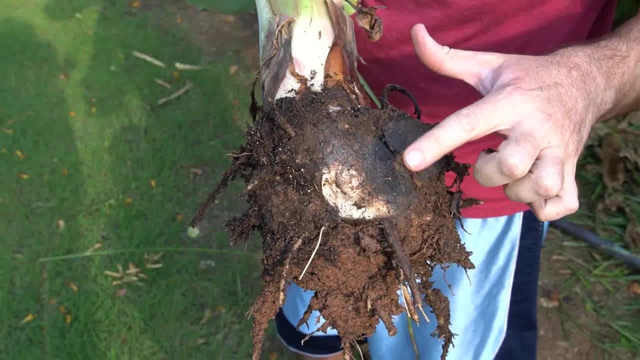 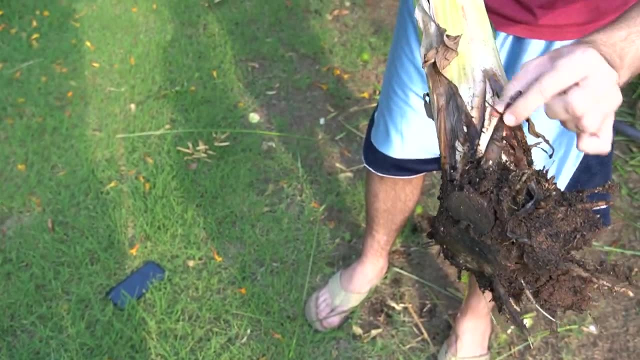 connected to the corn. it was connected to the mother plant, that underground system, and then you can see all the roots. it was trying to send off on its own and actually if you look here it looks like this: at one point was trying to be a pup, but it looks like it rotted. 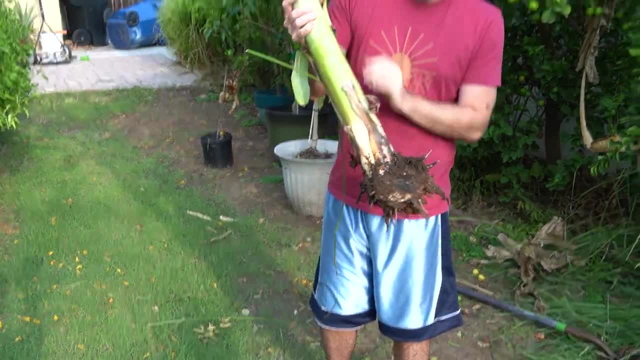 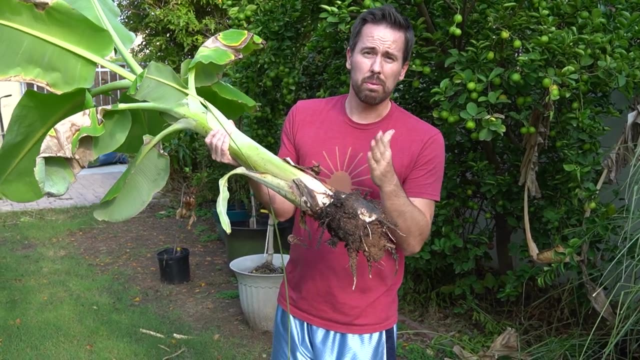 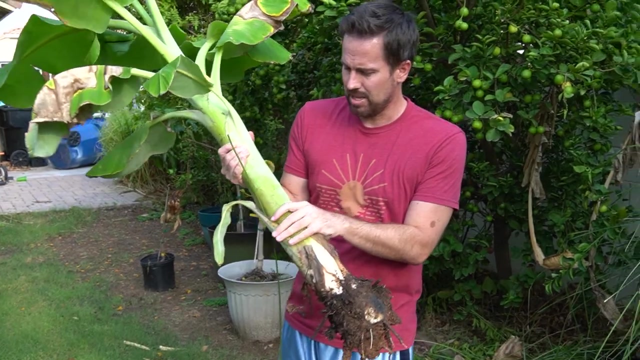 so at this point I'm not gonna show you how I plant it, because I have many other videos about planting. but remember, like with all trees, everything else you plant, don't plant it too deep. you don't want to plant it deeper than it was initially in the ground. also one word of advice when it comes to bananas. they don't want. 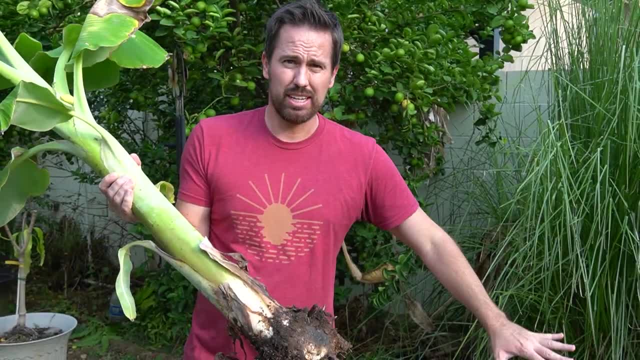 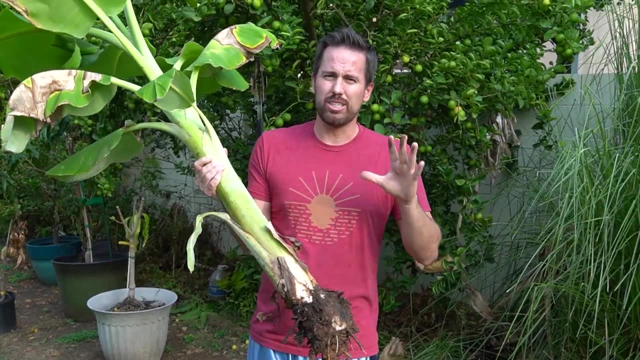 tons of water initially until they've had time to spread out their roots. these things are full of tons of water. if you give them too much water, they will rot. so once you initially plant it, you're gonna have a lot of roots and you're gonna have to keep it moist. don't let it dry out, but don't water it too much, or 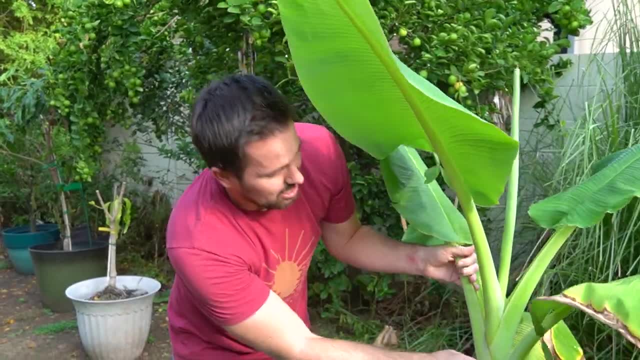 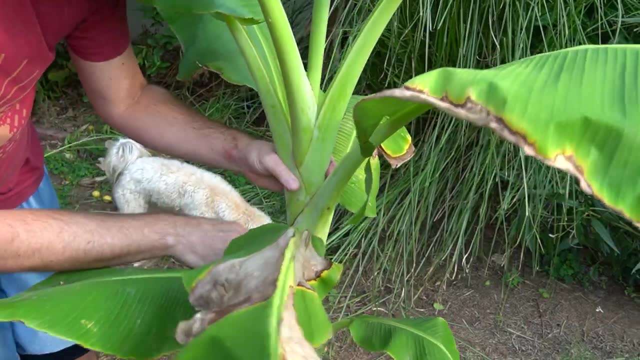 else it will rot. one other thing that I'm gonna do before I plant it is: I am going to cut off all of these leaves, every single one. I'm gonna cut off. that is because I don't want the banana plant now that it's not connected to the 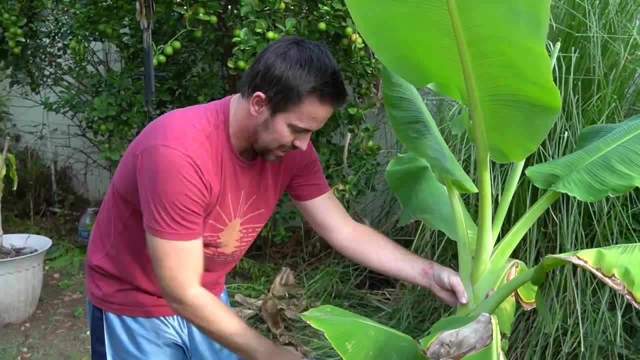 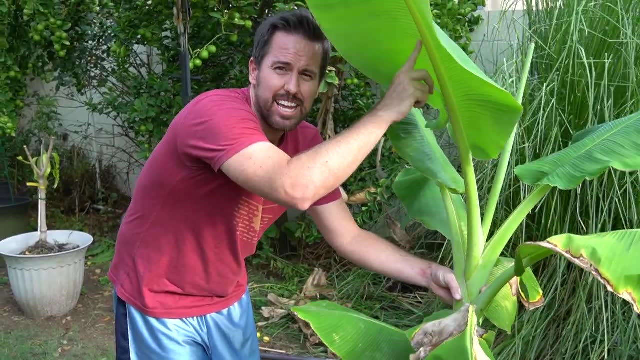 mother corn and it doesn't have that system feeding it and supporting it and it's gonna have to start spreading out its own roots and growing for itself. initially, I don't want it having to give nutrients and energy to the plant, so I'm going to cut off all the leaves, then we're gonna plant it and with time the